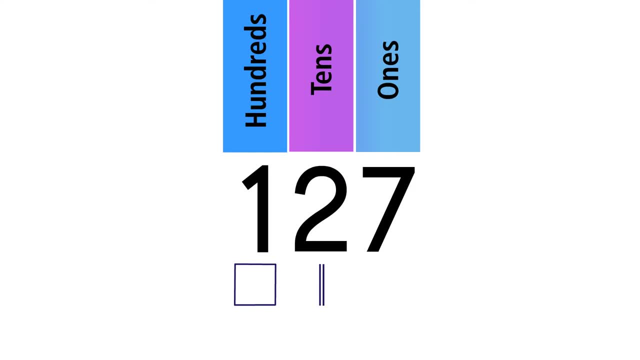 place, so we draw 2 bars. 1 bar represents 110.. We have a 7 in the ones place, so we draw 7 circles. A circle represents a 1.. We see that the 3 numbers are in different places and have different values. 1 has a value of 100,, 2 has a value of 20, and 7 has 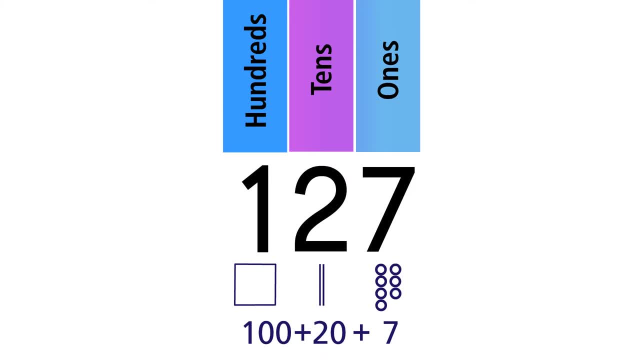 a value of 7.. When we add up all 3 values, we get 127.. Notice that each place is 10 times larger than the place to its right. We can easily see this when we put the same number into each place. 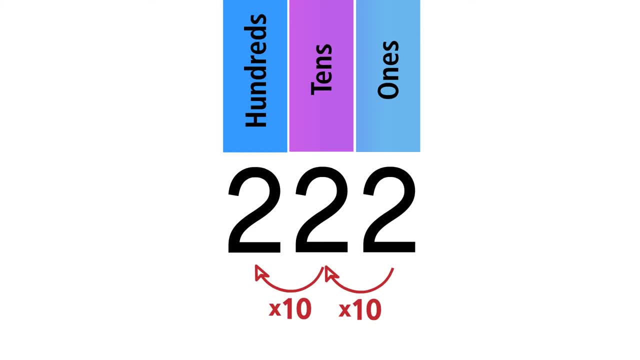 We have a 2 in the ones place, a 2 in the tens place and a 2 in the hundreds place. A 2 in the ones place has a value of 2.. A 2 in the tens place has a value of 20.. 20. 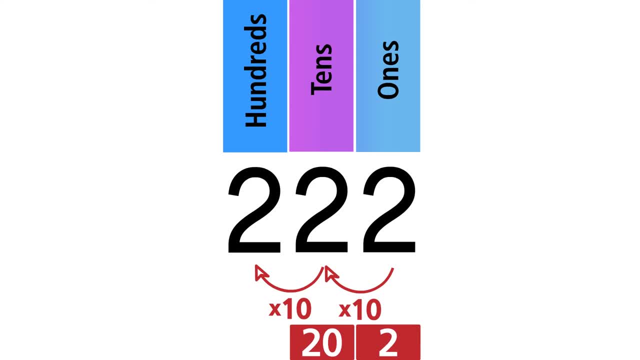 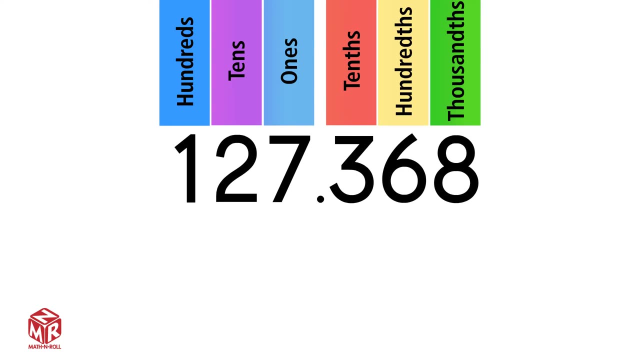 is 10 times more than 2.. We have a 2 in the hundreds place, so the value is 200.. 200 is 10 times more than 20.. Now let's take a look at Decimal Place Value. A decimal number consists of two parts: A. 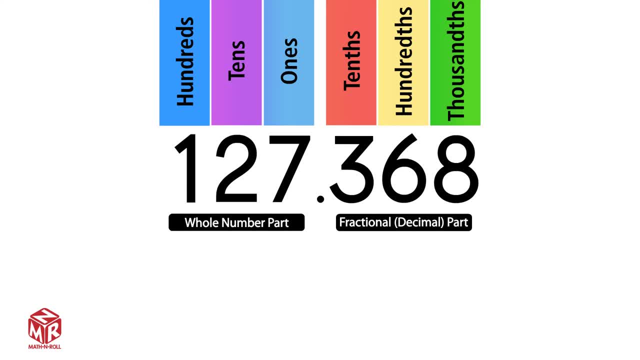 whole number and a fractional part. The whole number is to the left of the decimal. It can have ones, tens, hundreds, thousands and so on. The fractional part is to the right of the decimal. It can have tenths, hundreds, thousands, and so on. The fractional part. 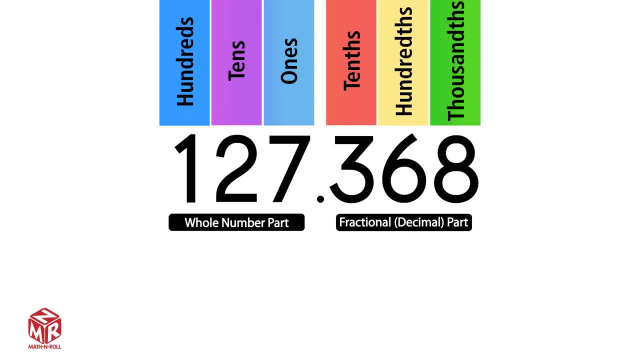 of the decimal represents parts of wholes. This part is always less than 1.. 1 tenth is the same as 1 out of 10 parts. 1 hundredth is 10 times less than 1 tenth. 1 thousandth is 1 part out of 1000 parts. 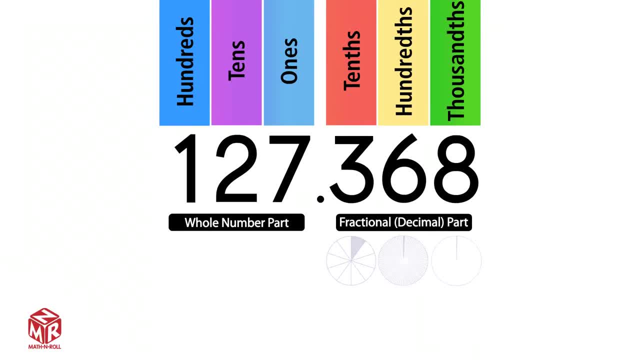 And it is 10 times less than 1 hundredth. The place values of the fractional part of the number end with th. So we say tenth, hundredths and thousandths. To start, let's remove the hundredths and thousandths. 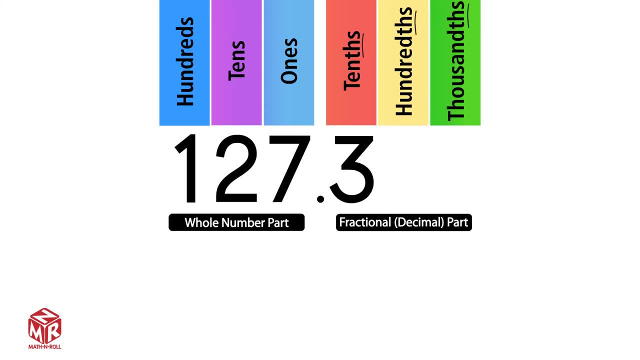 We have the number 127.3.. Let's draw it out. We have one hundred two tens seven ones and three tenths. Three tenths is the same as saying 3 out of 10 parts, So we split a. 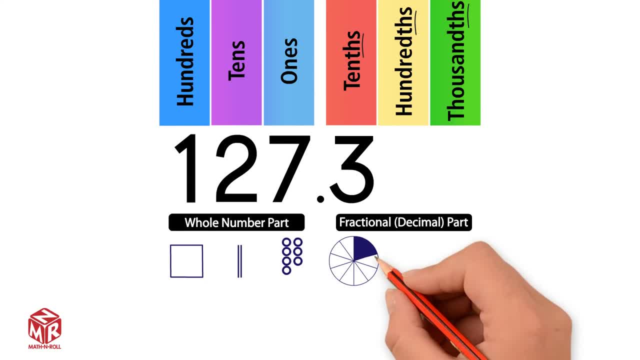 circle into 10 equal parts and shade in 3 parts. One hundred is the same as one hundred. Two tens is the same as 20.. Seven ones is the same as seven. 3 tenths is the same as 3 over 10.. When we add up these values, we get 127.3.. 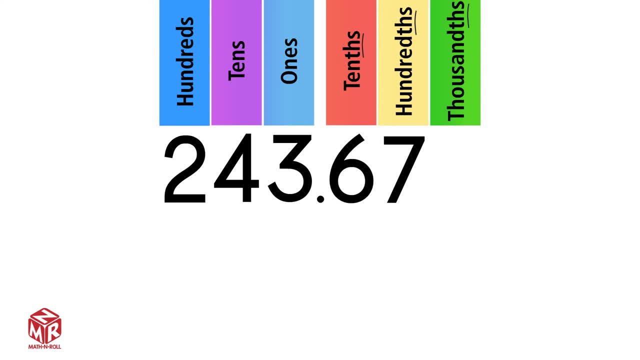 Let's try another example. We have 243 and 67 hundredths. Let's draw it out. We have 2 hundreds, 4 tens, 3 ones, 6 tenths and 7 hundredths. 6 tenths is the same as. 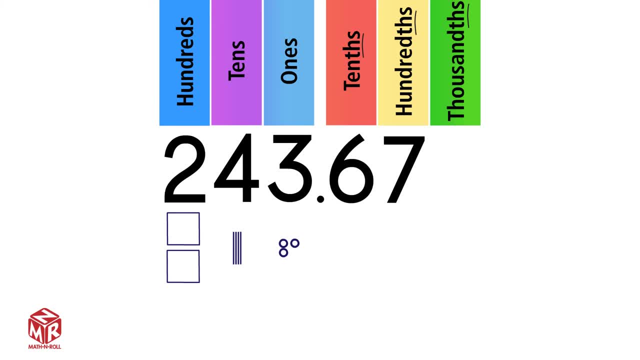 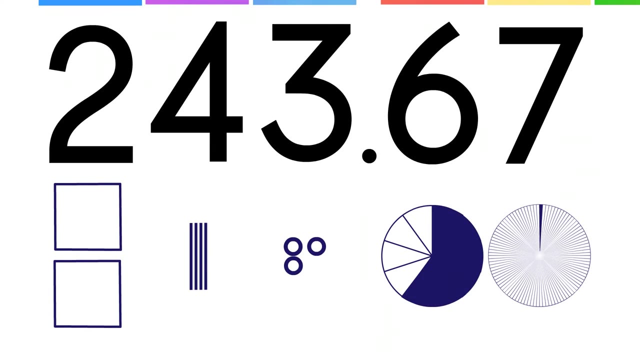 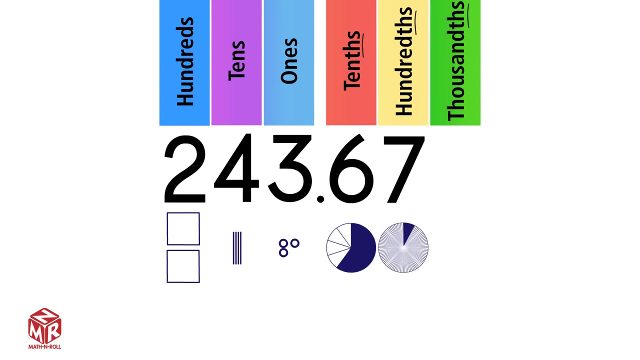 saying 6 out of 10 parts. We can draw 6 tenths by splitting up a circle into 10 equal parts and coloring in 6 parts. Now let's take a look at the hundredths. 7 hundredths is the same as saying 7 out of 100 parts. We can write 243 and 67 hundredths in expanded form. 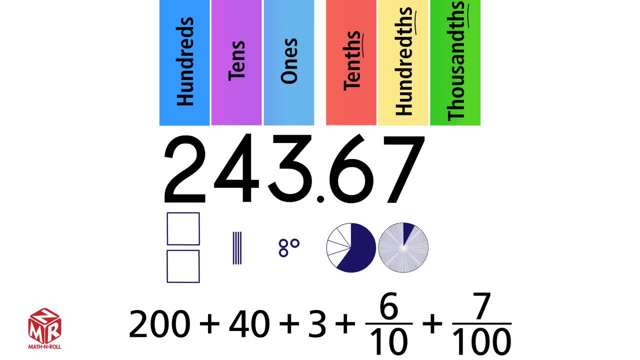 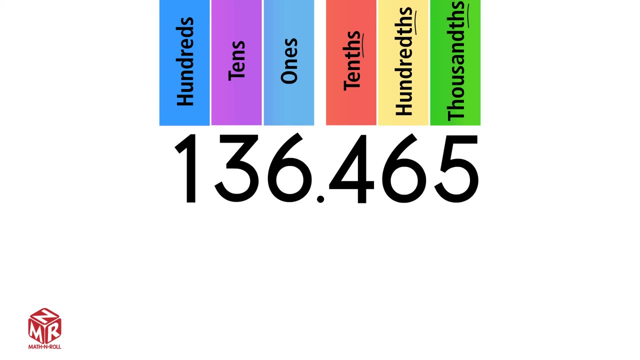 We'll have 200, plus 40, plus 3, plus 6 over 10,, plus 7 over 100.. Let's do another example: 136 and 465 thousandths. Let's draw it out: We have 100, 3 tens 6. 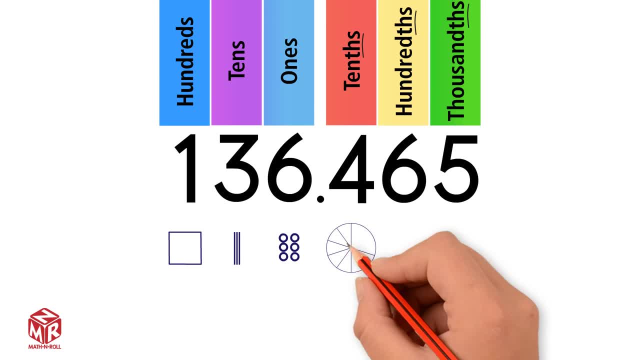 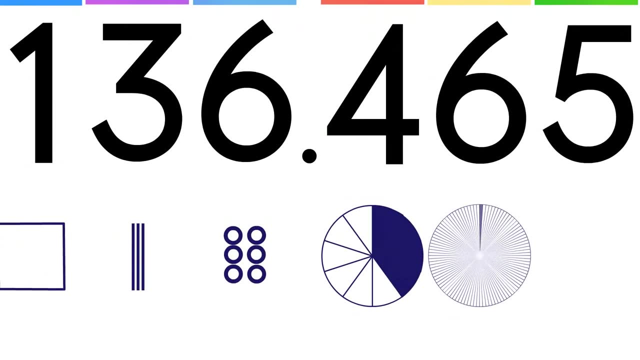 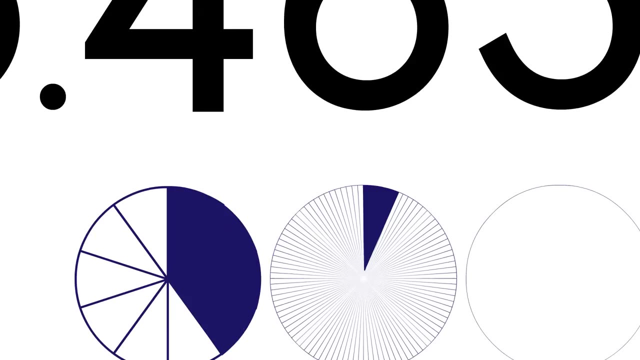 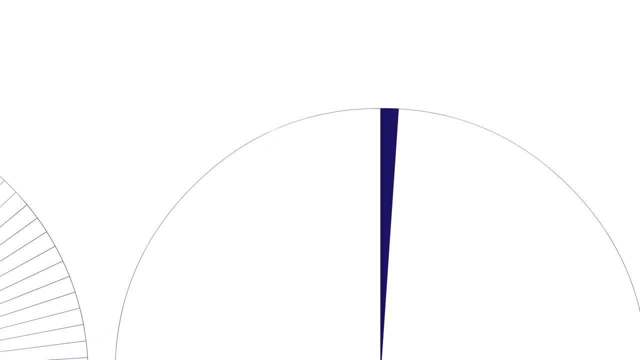 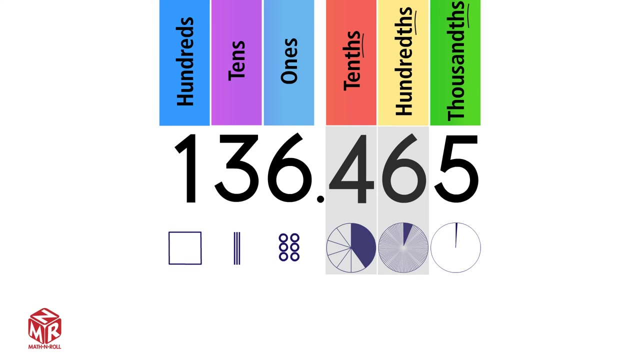 ones: 4 tenths, 6 hundredths and 7 hundredths. We can add up these values And 5 thousandths. Let's draw 10 thousandths again: 4 tenths is 4 out of 10,, 6 hundredths is 6 out of 100, and 5 thousandths is 5 out of. 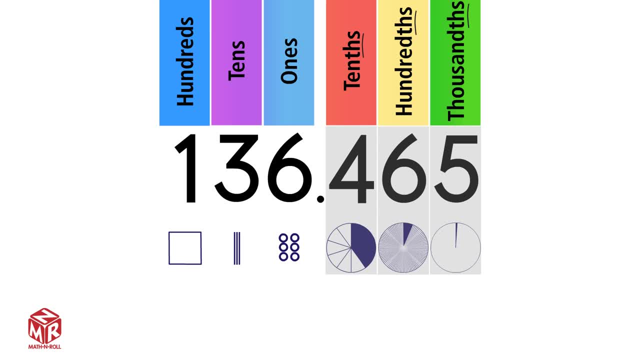 1,000.. Let's write the decimal number into expanded form. We've added in the decimal numbers. Let's draw the next one. We have 100, plus 30, plus 6, plus 4 over 10, plus 6 over 100, plus 5 over 1000.. 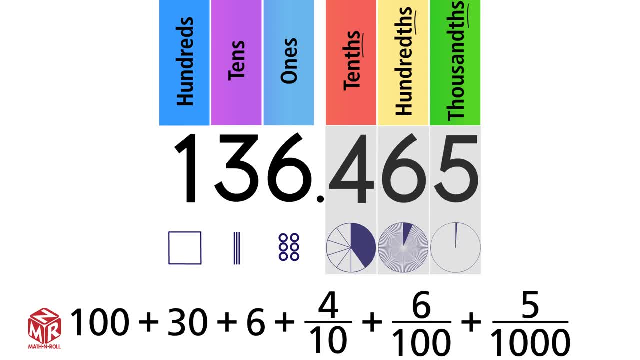 If you thought this video was helpful, please leave a like. For more videos like this. please subscribe.